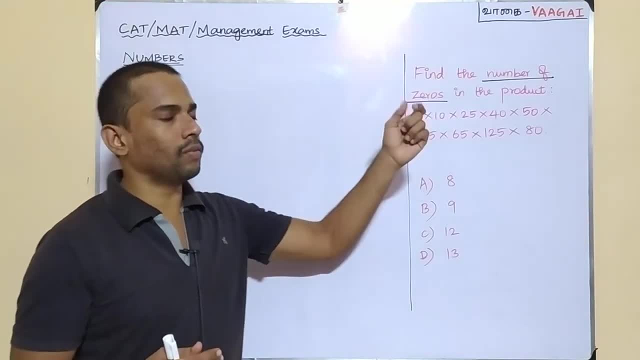 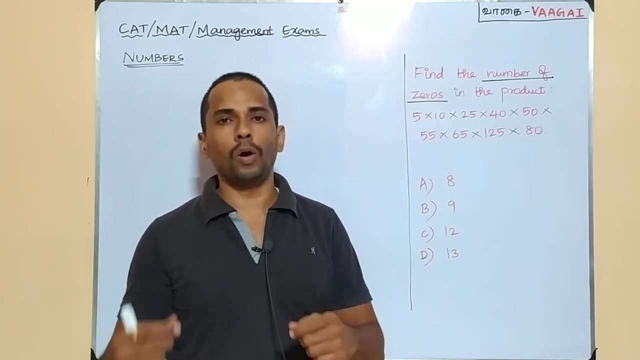 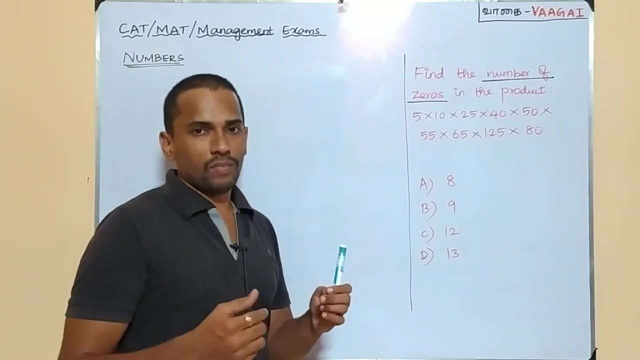 The question is: find the number of zeros in the given product. So the question is asking for: find the number of zeros. If you remember, we have already worked few problems based on the same idea: find the number of zeros. So what we do there actually? So whenever we need to find the number, 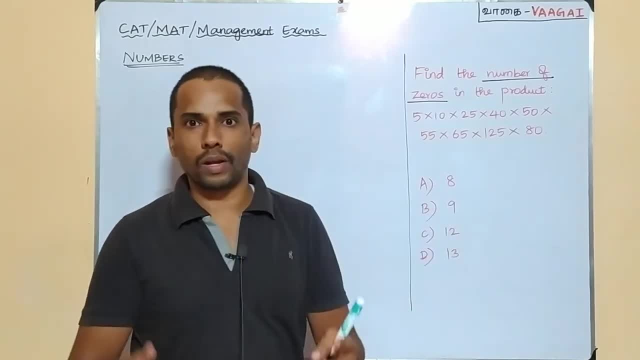 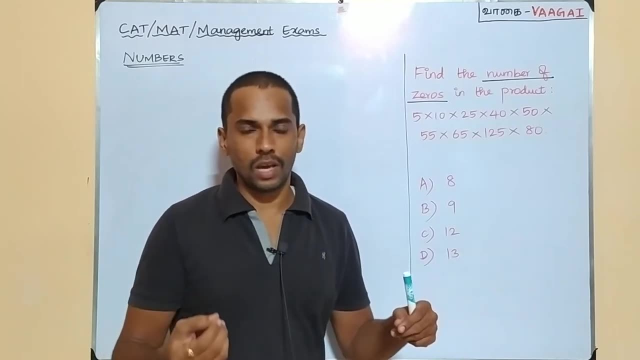 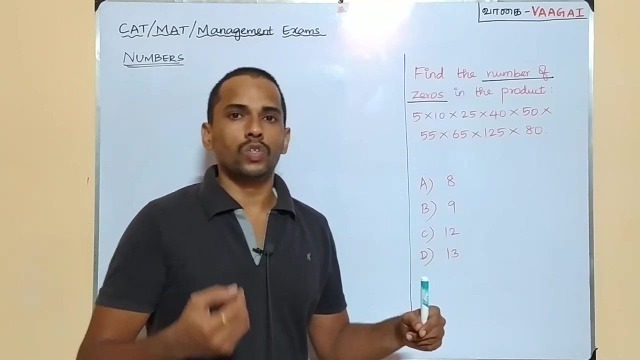 of zeros for a given factorial or for a given product, whatever given. So what we try to do there is we will be collecting the tens there, Tens because you know each zero there in our number represents one, one ten. that is the reason. Okay, so, for convenience, what I will do is I will attach the link of those videos here in the 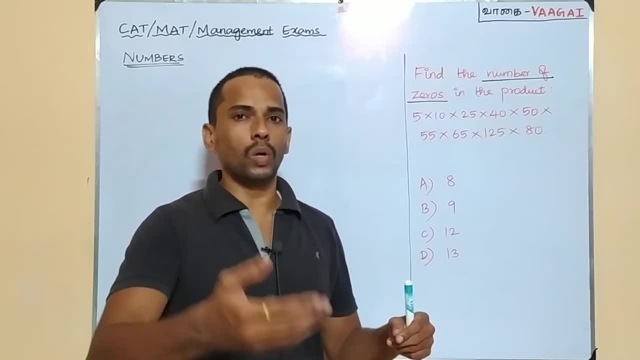 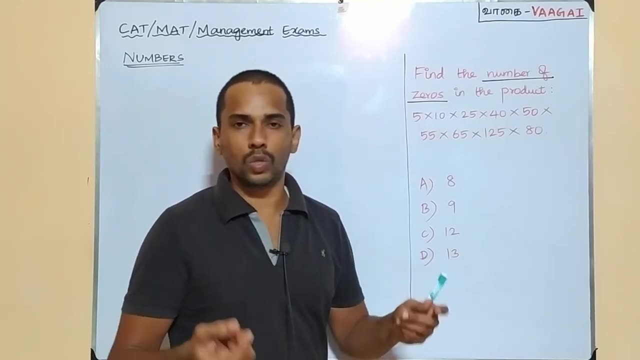 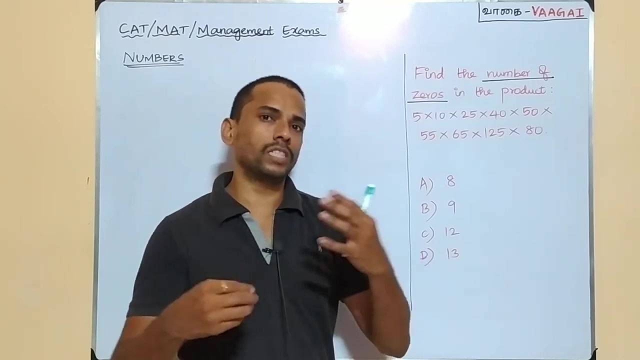 description box of this video so that it will be easy for you to refer those videos. Yeah, coming back. so one zero. if there is one zero, that means it represents one ten. So that means our idea here is we need to find how many tens are there, or maximum, what? what is the maximum power of ten? 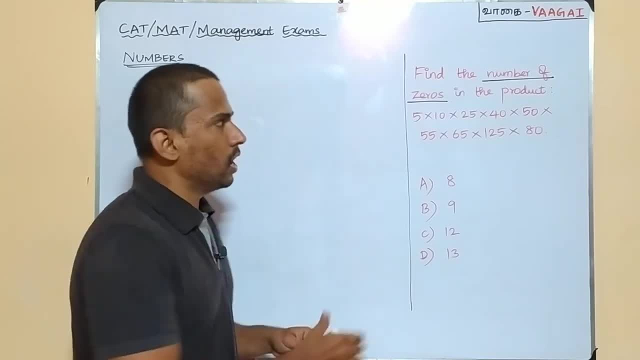 available in our given content. that is what we have to see. Okay, so the moment you see the number of zeros in the question, Okay, so that means we have to find the number of zeros in the question. So that means we have to find the number of zeros in the question. So that means we have to find the number of zeros in the. 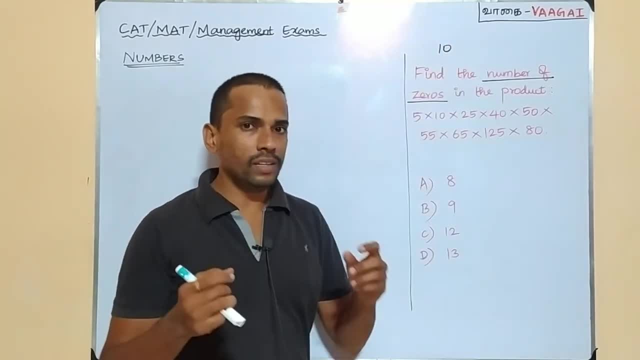 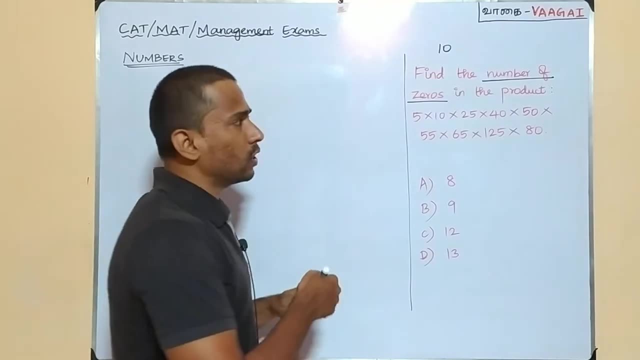 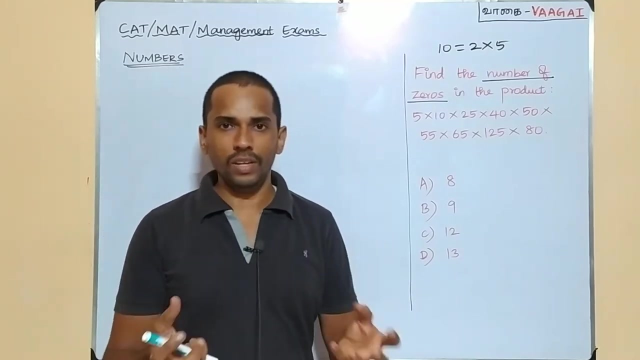 given product. Okay, this is what we have to check. and what about ten there? To get one ten, again what we have to see. just try to decompose the number ten. Okay, so this ten can be written as what It can be written as two into five. Okay, so correct, as many twos and fives in our given. 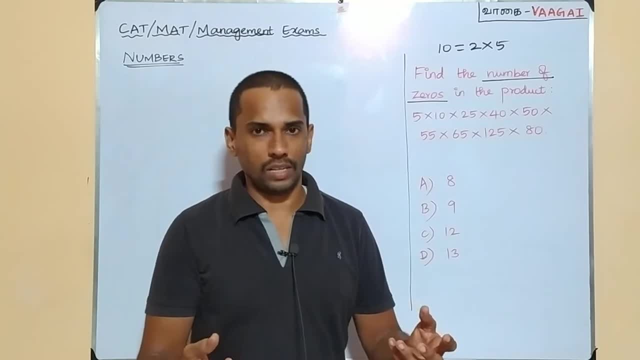 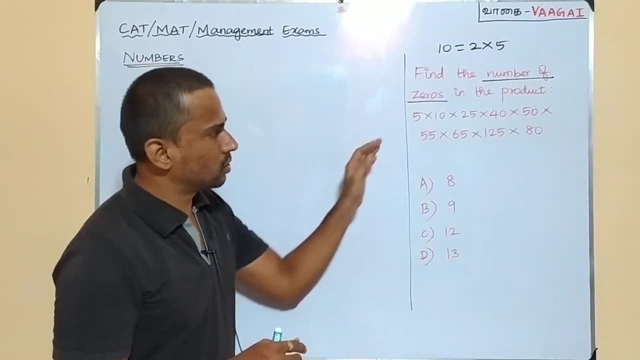 expression, So that will easily give you the answer. That's it, Okay and yeah. coming here to the question: find the number of zeros in the given product. and what is our product? Our product is appearing to be little lengthy, So that means we have to find the number of zeros in the given. 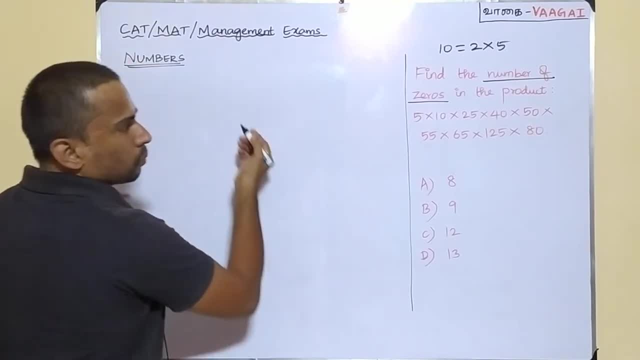 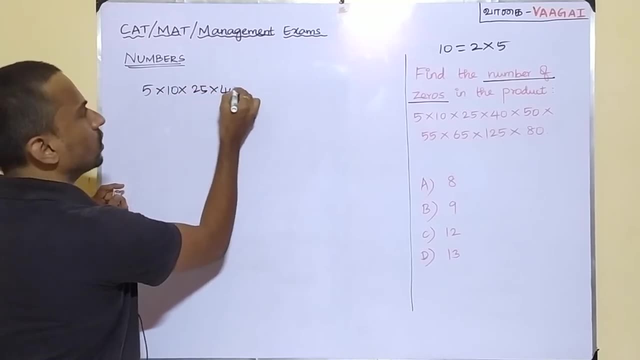 So we will find the number of zeros in the given product. and what is our product? Our product is lengthy, Anyways, we'll just take it down here. So the product given here is 5 x 10 x 25 x 40 x 50. 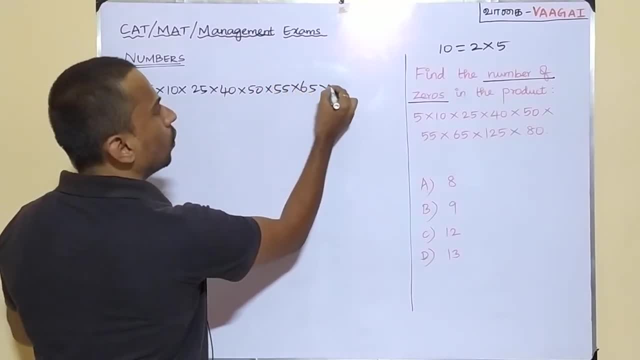 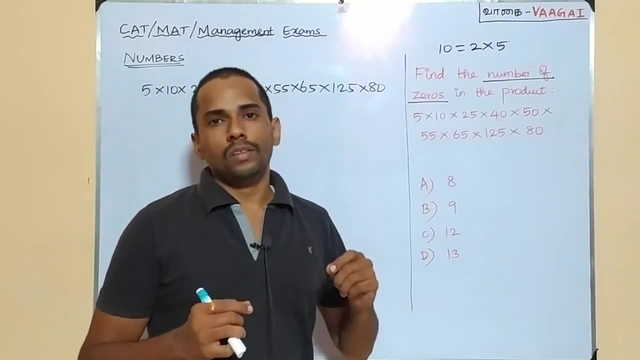 multiplied by 55 x 65 x 125 x 80. So, of course, a very long product we have here. So, for this product, this will have how many zeros at the end? This is going to be the equation. Okay, all right. 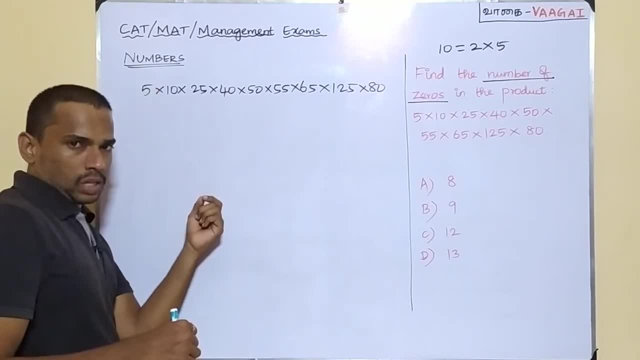 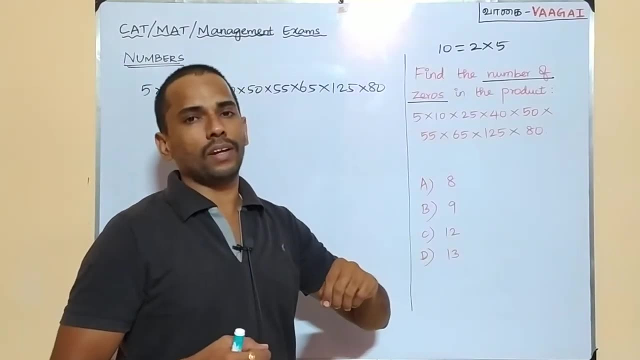 So now what we will try to do is we will try to decompose the number in terms of 2s and 5s. Why 2s and 5s? Just now we saw the reason, because the reason we need to get collect as many 10s possible. 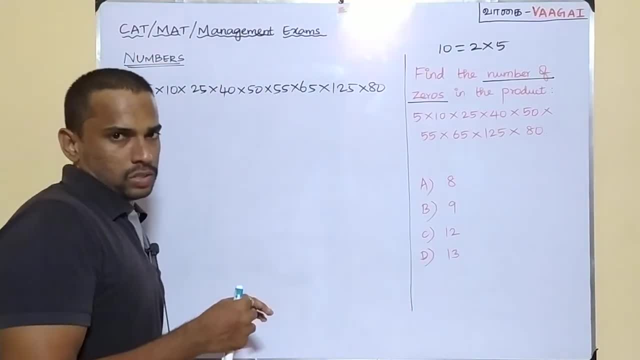 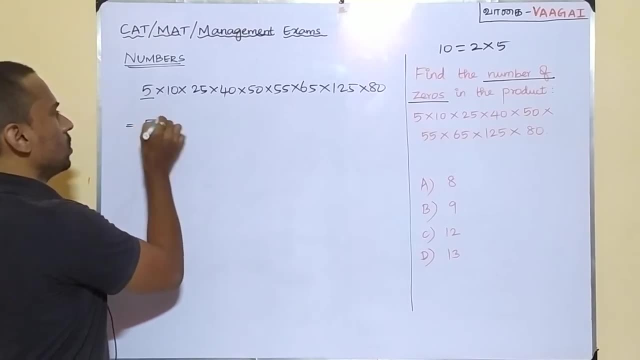 for that. only, we are doing this, okay, So now break each of these numbers. let us try to do that. so start with this 5, okay, So this 5 can be simply written as what 5? only right, so 5, so it is like 5 power 1, okay, let me write like that. 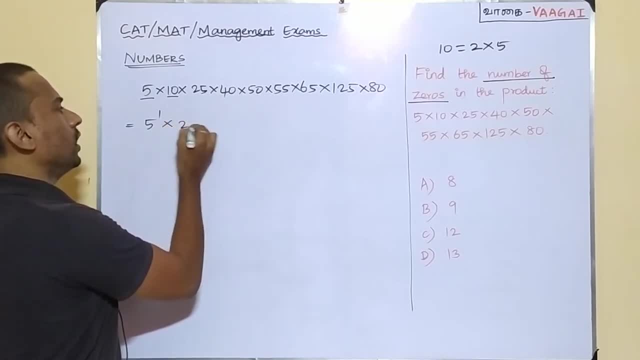 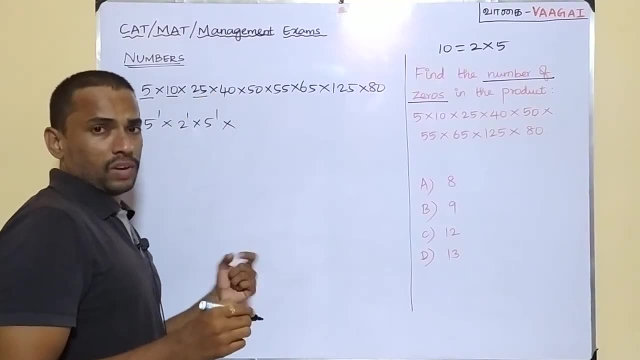 Next, this 10 can be written as what. This 10 is once again 2 into 5, or I can tell: 2 power 1 into 5, power 1, okay, over multiplied with. next comes this 25, 25 can be written as what: 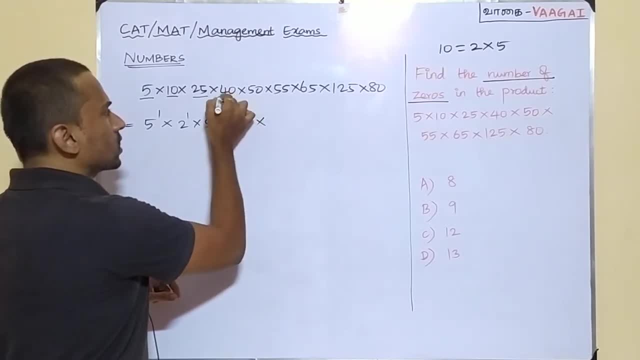 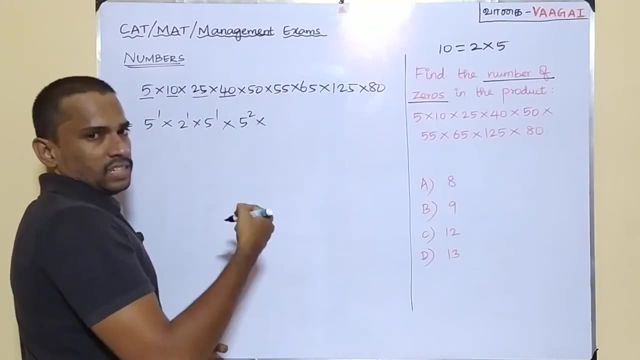 This is nothing but 5 square, is it or not? Yes, multiplied by next comes this 40, this 40 is actually what? 40 is actually? 8, 5s or 40,, is it or not? So that means this 40 can be written as 8, that is, 2 cube multiplied by 5, so I hope. 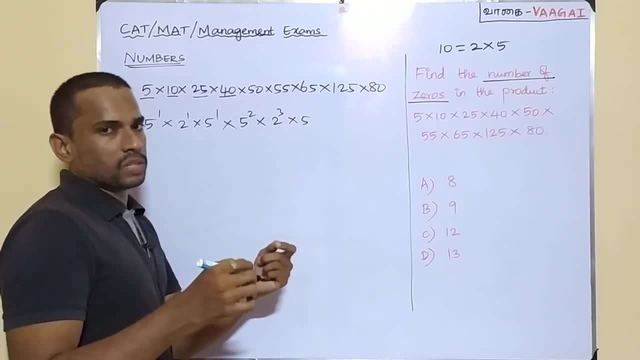 you are able to follow that? okay, I am trying to rewrite the numbers in terms of 2s and 5s. Yes, wherever possible. that is it, okay. Next, coming to this 50,. what about 50,? 50 can be written as what? 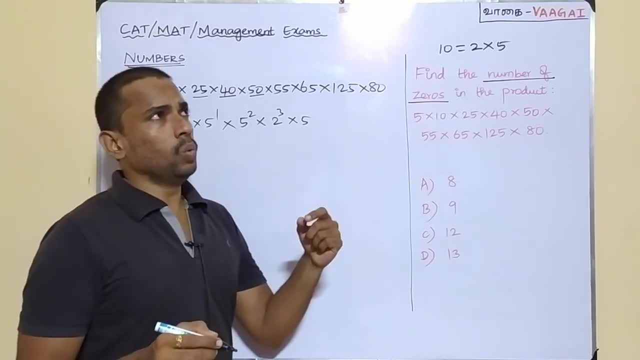 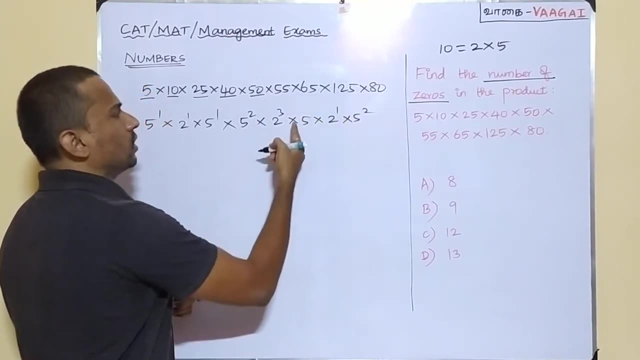 50,. inside that 50, we have 2 and 5,, is it or not? So that means this 50 can be written as 2 power 1 into 5 power 2, okay, So here this is like 5 power 1,. okay. the previous thing. 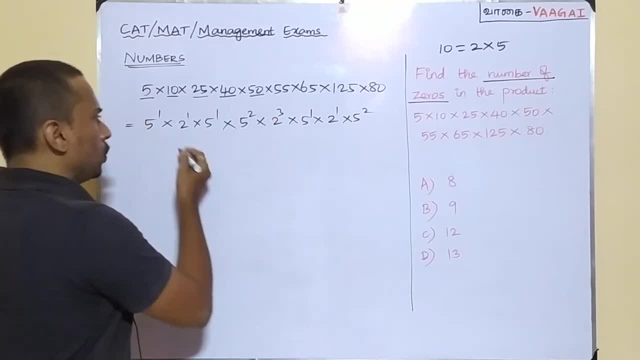 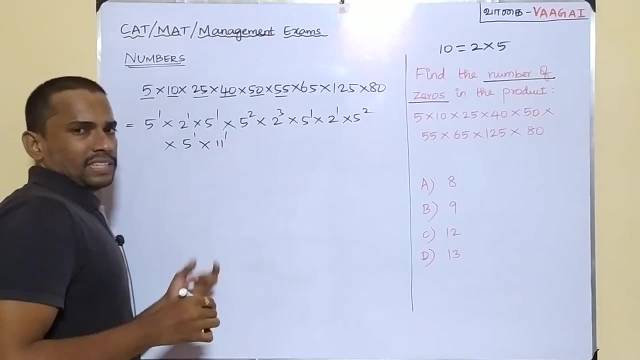 So 2 power 1 into 5 power 2, that is what is this? 50,- yeah, I am continuing down- multiplied with this 55, next number is 55,. 55 can be written as 5 power 1 into 11 power 1, anyways. 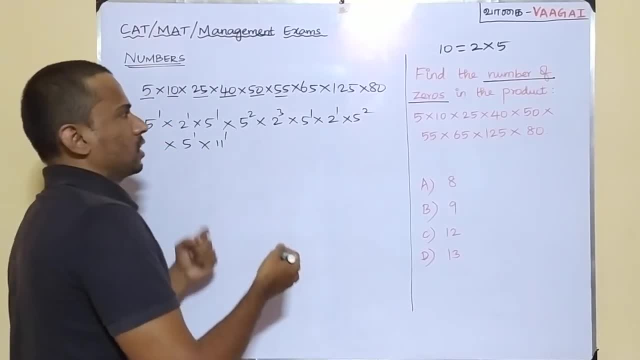 11s. we do not need, but still, I am just taking it as expression, okay. Next, we have 65, this 65 is nothing but 5 power 1 into 13 power 1, because 65 is nothing. 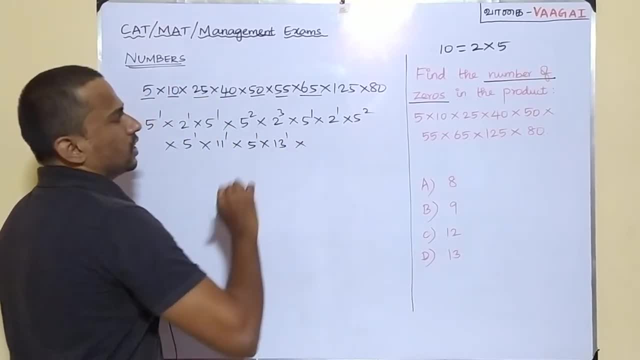 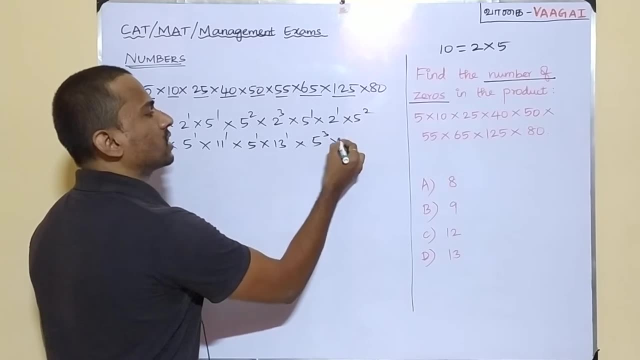 but 5 13s, all right. So yeah, continuing it. next we have 125, so 125 is exactly 5 power 3, right, so 5 power 3. and next last one, we have 80, so this 80 can be written as what: 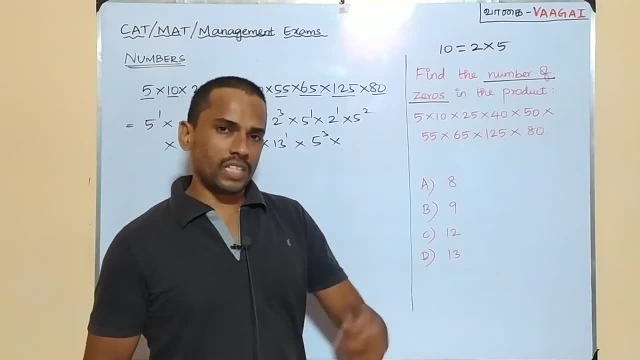 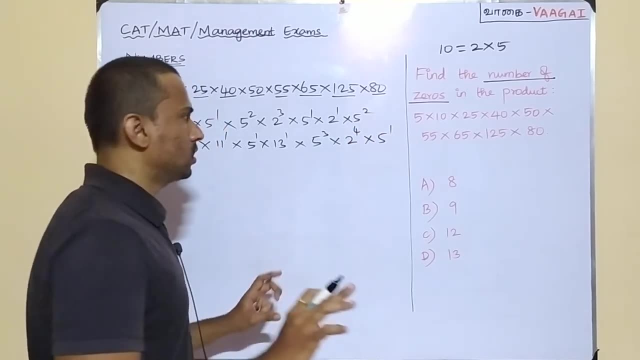 80 is nothing but 16. 5s are 80, right. So once again, that 16 can be written as what? 16 is nothing but like Now: 2 power 4 multiplied by 5 power 1, I hope you are able to understand this. 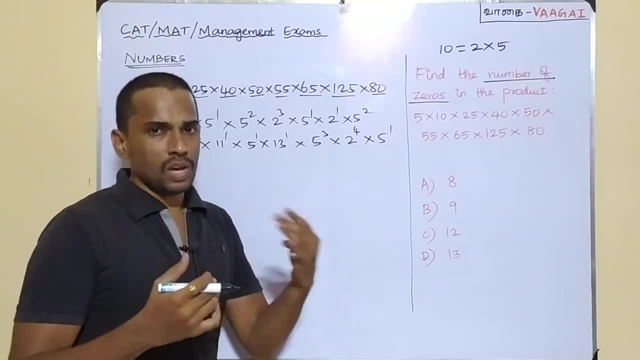 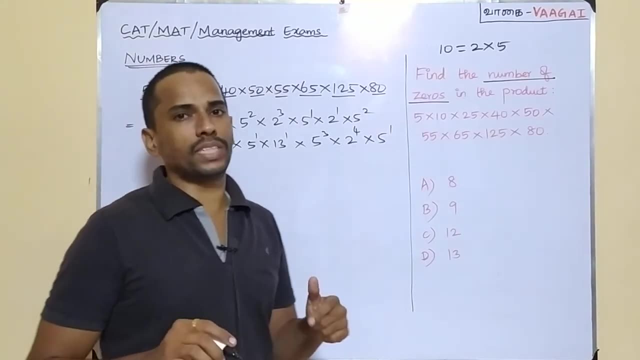 So now, clearly, we have decomposed these numbers in terms of powers of prime numbers. that is it, very simple. okay, Now what we need to do here is we have to collect 2s and 5s alone. why 2s and 5s alone? 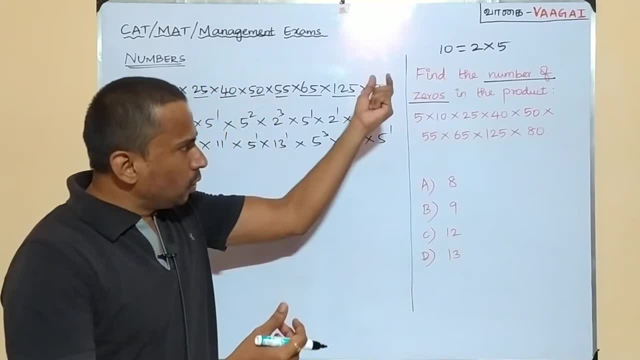 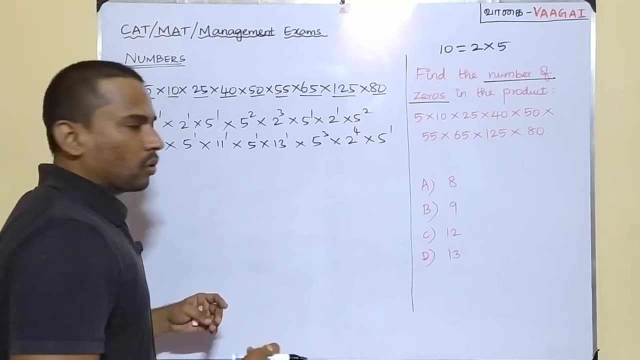 Because all we are worried about is here. we are just worried about only the number of 10s here, so that means we it is enough for us to collect only the 2s and 5s. let's try to do that, okay. 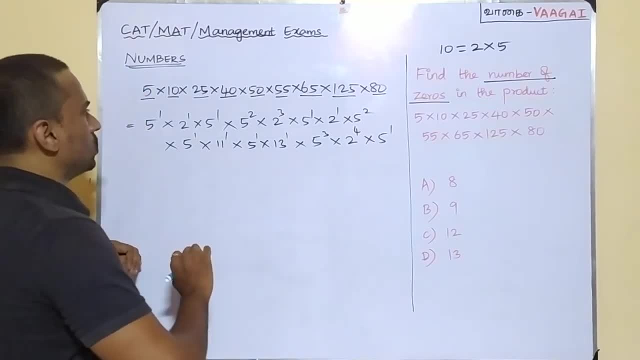 So now coming with the 2s. okay, so whatever 2s, if you see, wherever 2s you have, you can pick them. so here we have 2 power 1, okay, so 2 power 1 you have here or we can directly. 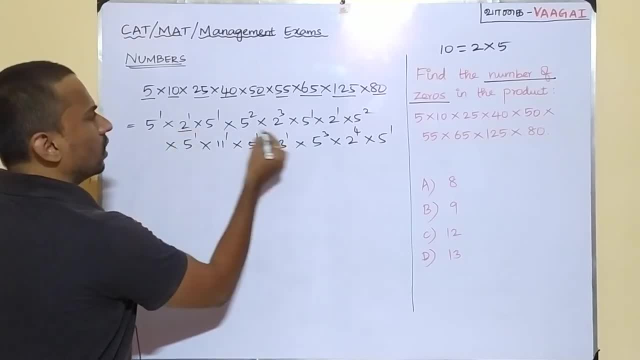 count it as it is okay: here we have 1,, next we have, here we have 3, right, so that means 2 power. we have 1 plus here 3, and next we have plus 1 and next 2 is where where we. 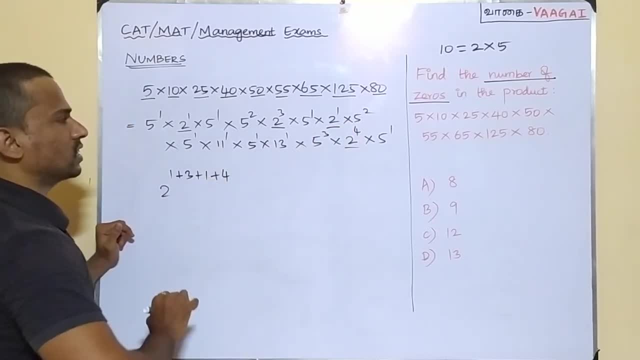 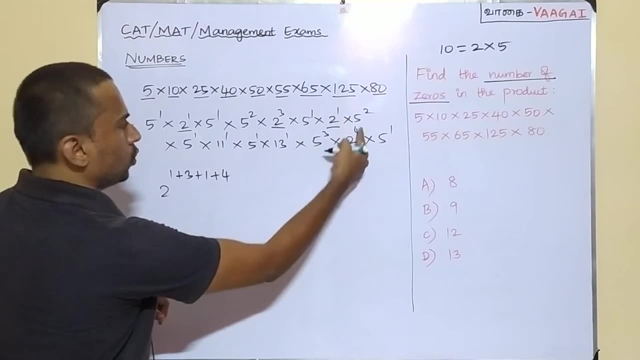 have 2s. here is another 2, right, so plus 4, so that's it okay Here here, here, here, there are only 4 expressions with 2, so 2 power 1, 2 power 3, 2 power 1,. 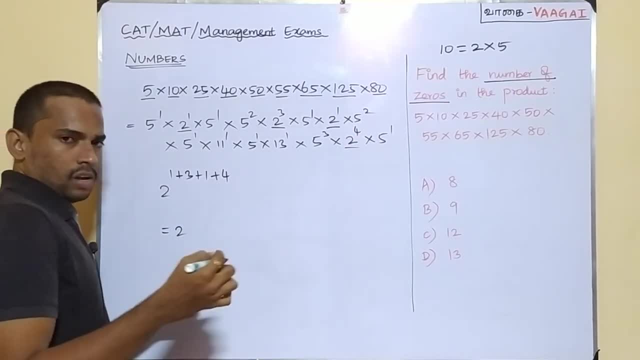 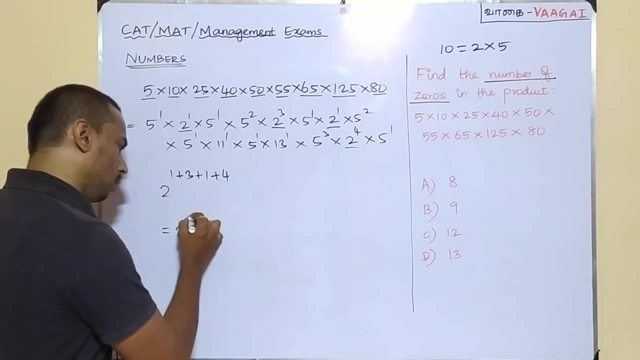 2 power 4, so that means they all come together, or they all they get multiplied together and totally we will have what 1 plus 3 plus 1 plus 4, which will give us how much. this will be nothing but 2 power 9,, is it or not? yes, fine. 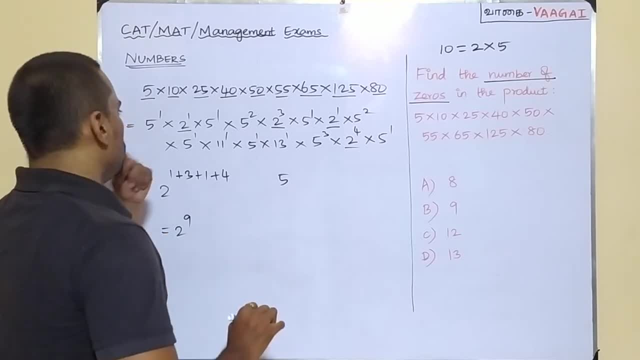 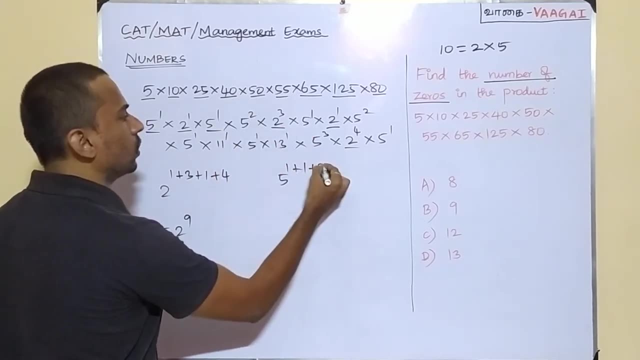 Next come to 5s powers. so coming to 5s powers, here 5s powers will count to. here we have 5 power 1 plus again 5 power 1 plus here 5 power 2 plus here 5 power 2 plus here. 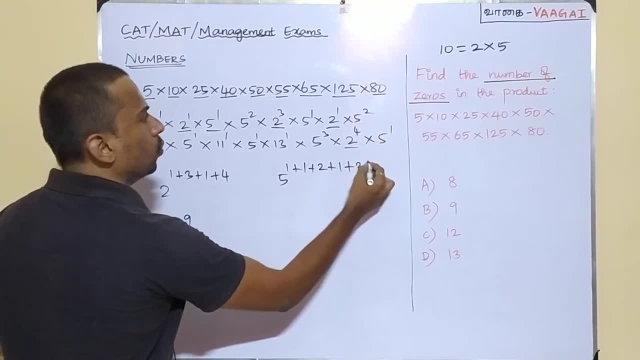 again 5 power 1 plus here 5 power 2 plus here, here, here over next 5 power 1, and then again plus 1, again we have plus 3 plus 1, so I am writing it as 4 together, because 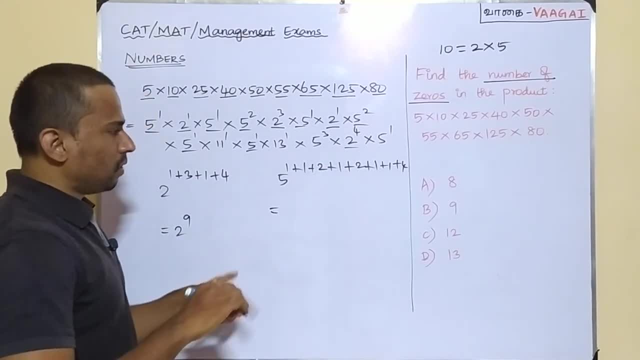 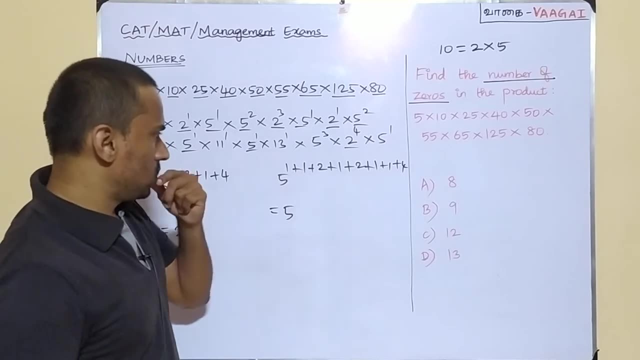 of. there is no space. that's the reason. okay, So it seems that 5 power is more available, right? 5s powers. we have a lot more 5s than 2s, that's the reason. so, anyways, if you see, let's confirm it. okay, so 1 plus 1, this. 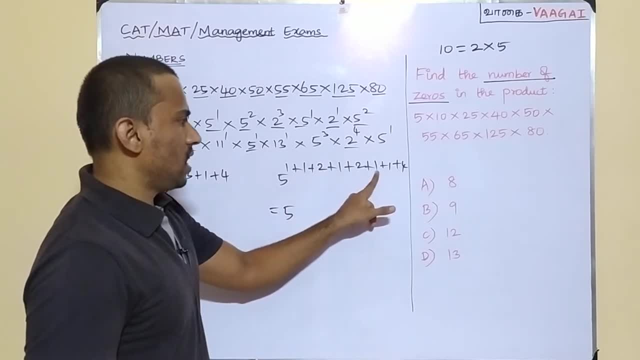 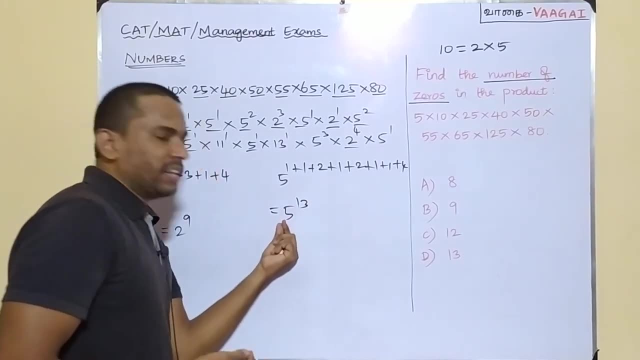 will be like 2,, 4,, 5.. 6,, 7,, 8,, 9,, 13,. so we have 13 5s. so that means there are 9 2s and 13 5s available. 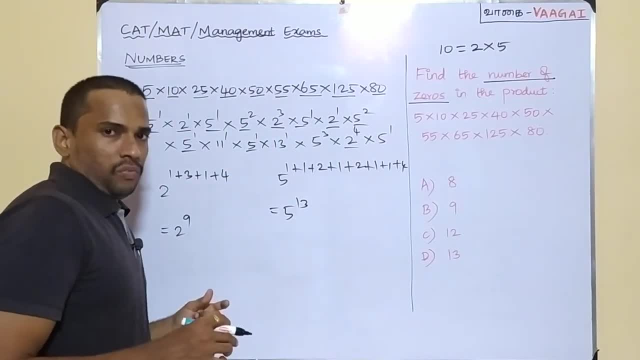 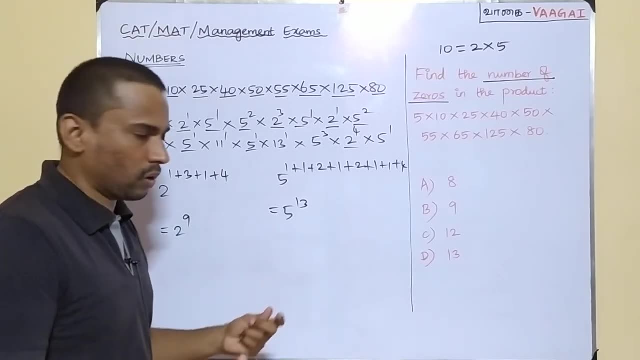 inside this product. that's the meaning. okay, Now just think of when we try to collide these terms: maximum, how many 10s can we form? that's what we have to think. okay, there are 9 2s available. that is 2 power. 9 means 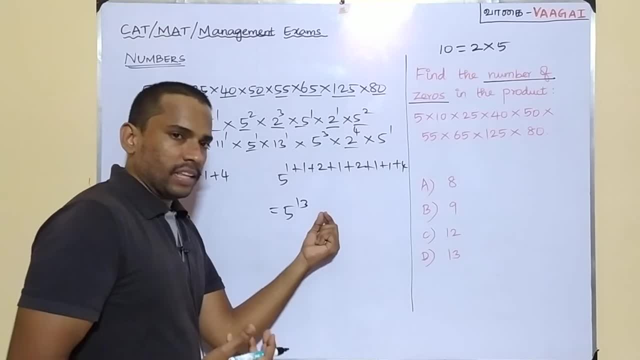 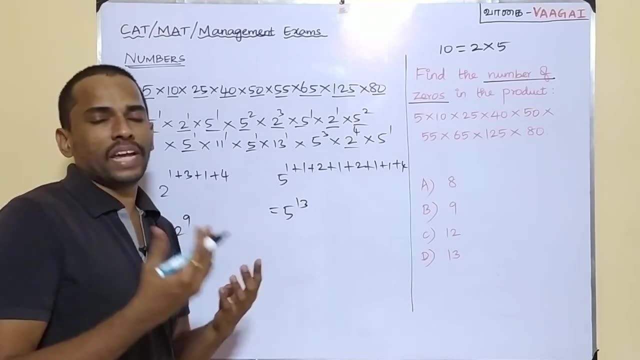 we have got 9 2s available and 5 power 13,. that means 13: 5s available. so when they make them to combine to form 10s maximum, how many 10s can be formed? that is what we have to think. so it's very. 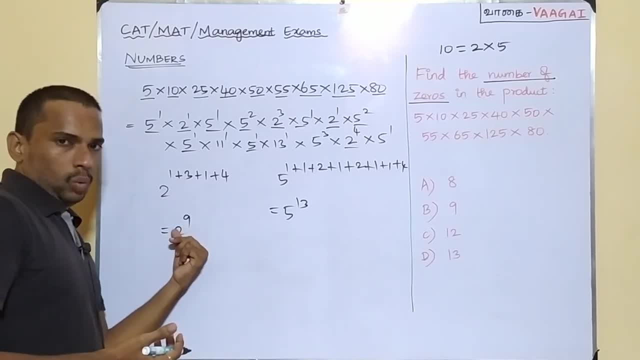 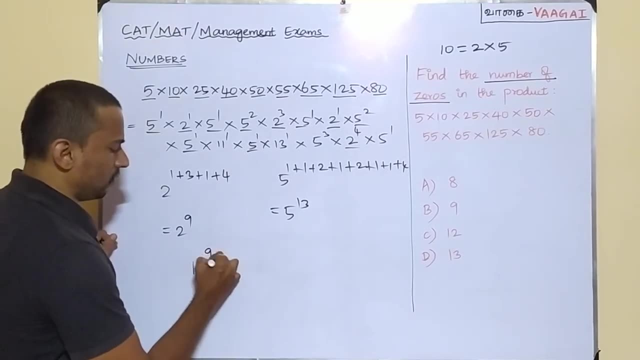 clear here: the least power is available with 2 only, which is going to be 9,. so that means at a maximum, at a maximum, we can collect only 9, 10s. that means 10 power, 9, okay so. 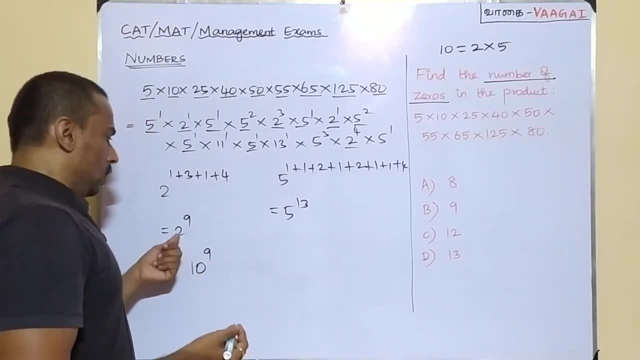 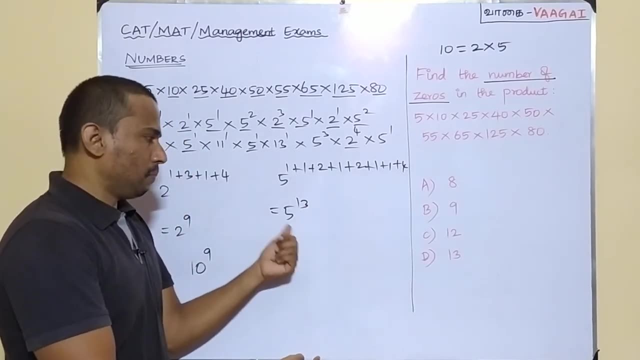 that means only 9 10s. we will be able to collect why: because 2 power 9 here will combine with 5 power 9, because the other 4 power- I mean 5 power, 5 power 9, when we just take this. 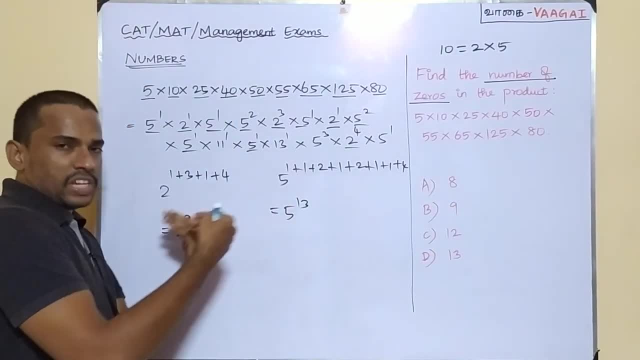 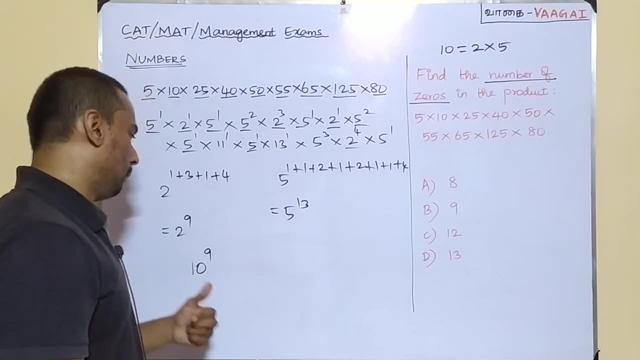 5 power 9, 5 power 9, the other 5 power 4 will not have sufficient 2s to collide to form 10, that is the reason. so 2 power 9 with 5 power 9 alone we can combine to get a maximum of 10 power 9,. so that means: 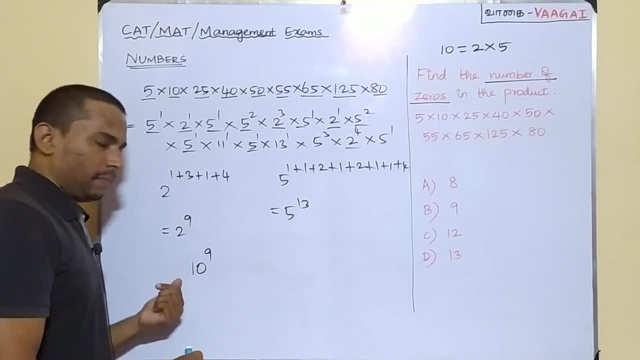 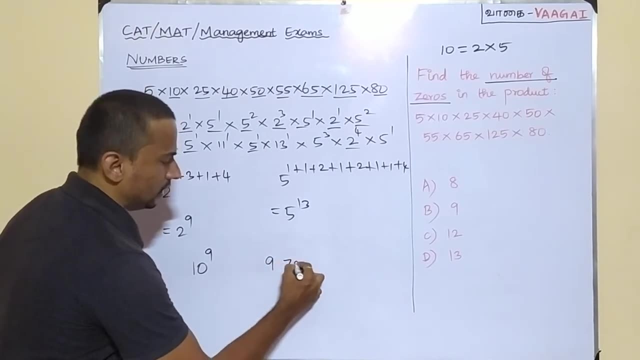 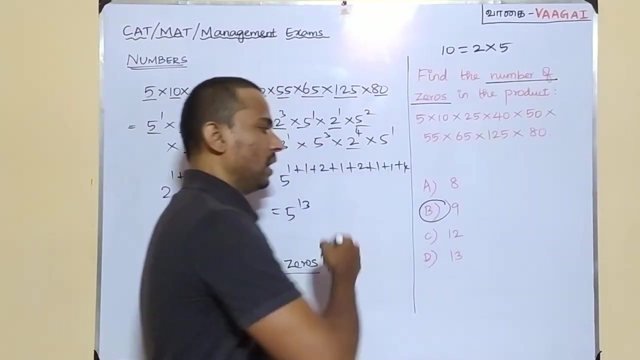 we can maximum collect 9 10s here. so that means our product will have how many 0s at the end. it will have 9 0s at the end and that is going to be the answer. okay, find this. so our answer. 9 is already available at option B. so option B: 9 is available at. 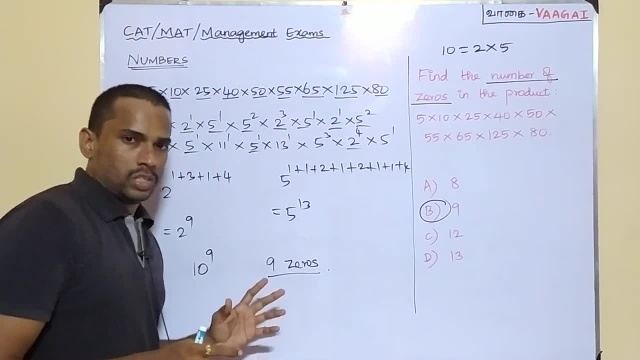 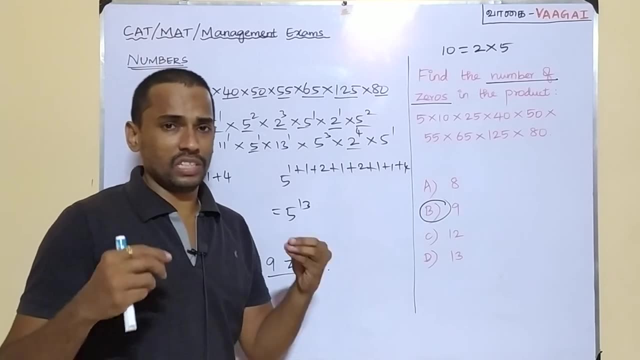 option B 9 is going to be the answer for this question. I hope you are able to follow this. so I won't say that this question is very difficult, very harder one. but the way students usually they prepare the aspirants when they see this question, they will consider. 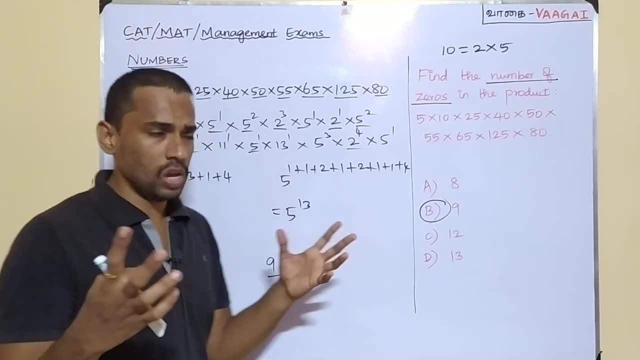 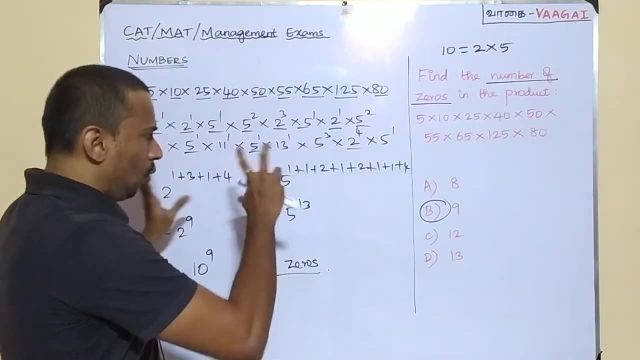 these questions to be harder, but the way of solving it is going to be very, very easy, okay, if I guess, though, I have given more explanations orally. if you are clear with the concept, it won't take more time for you to solve and get the answer. it's just a quick. 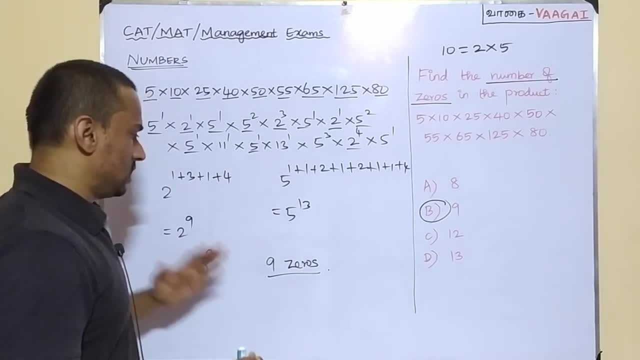 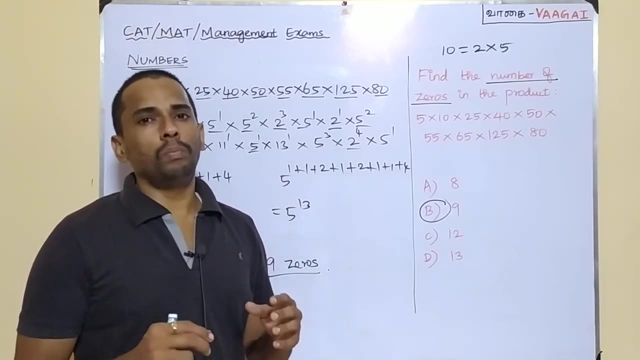 very simple process. you can quickly solve and then get the answer. yes, I hope you are able to follow it. 9, 9 is going to be the answer, which is option B is going to be the answer for this question, and I hope this session was useful to you and if you feel. 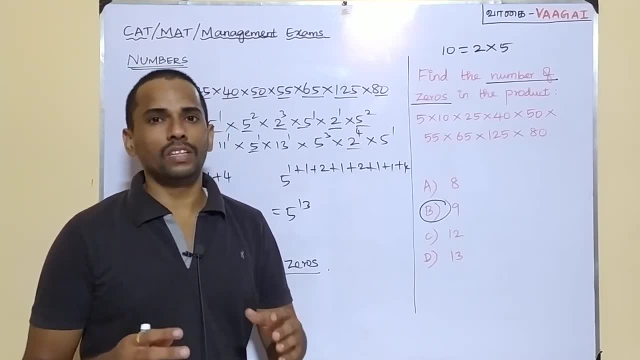 like this session was useful to you, please give a like and if you feel that this would help any of your friends, please do share this video to your friends also. and again, we will catch up in the next session with some other interesting question. see you soon. there. thank you so much.